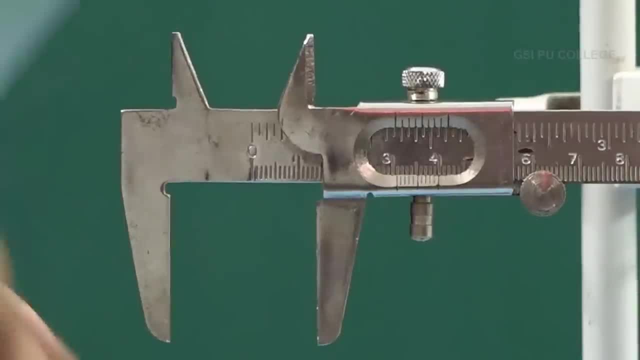 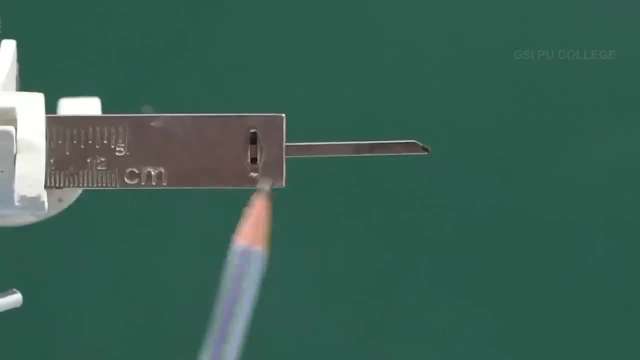 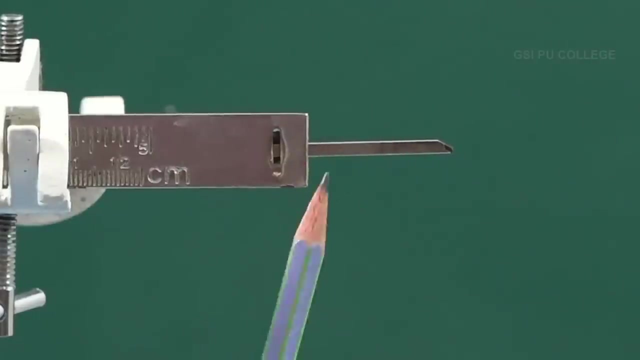 And these are called upper jaws. So upper jaws are used to find the internal diameter of a cylindrical object. So these are called upper jaws. So at the end you can find a strip. So this is also used to measure a length. This one is used to find the internal. 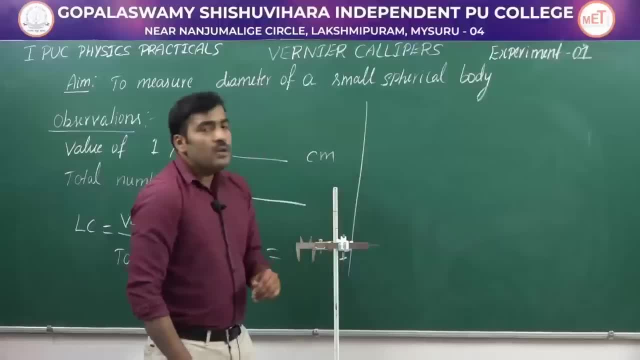 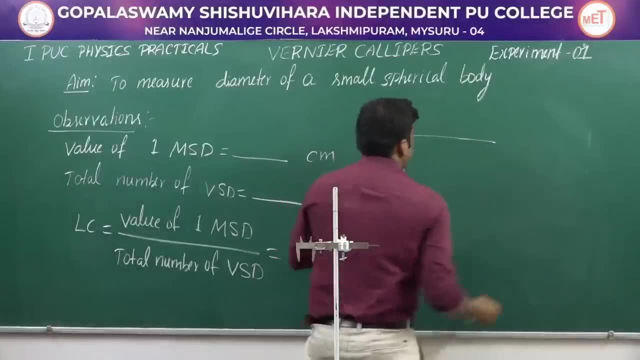 depth of the cylindrical body. Okay, Fine, See how are the divisions in the main scale. If this is a main scale, this division is the zeroth division. This is called as a zeroth division, And after this you find a ten divisions. 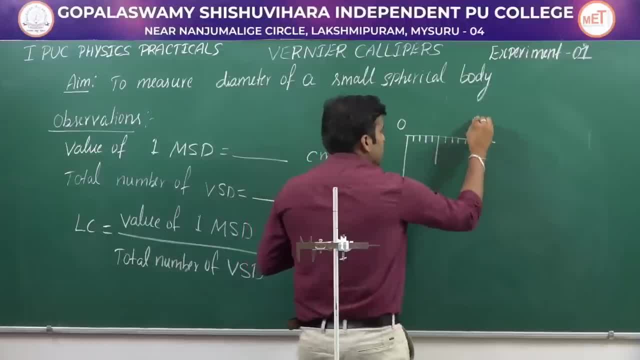 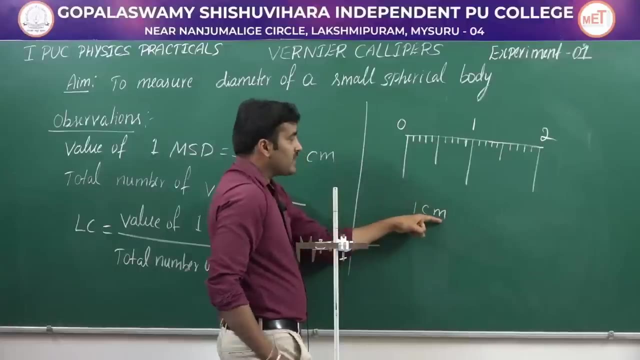 and here it is marked as one. Next, So in your main scale, the divisions are like this: In between this zero to one, we have one centimeter distance. From zero to one, we have one centimeter distance, and in between this one centimeter there are ten equal divisions. There are ten. 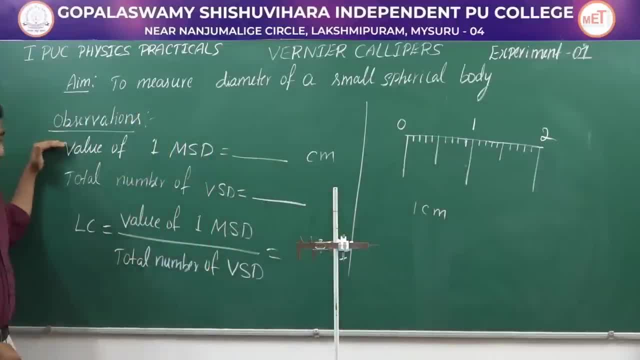 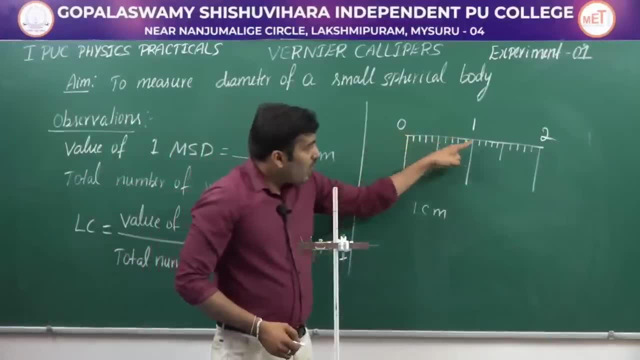 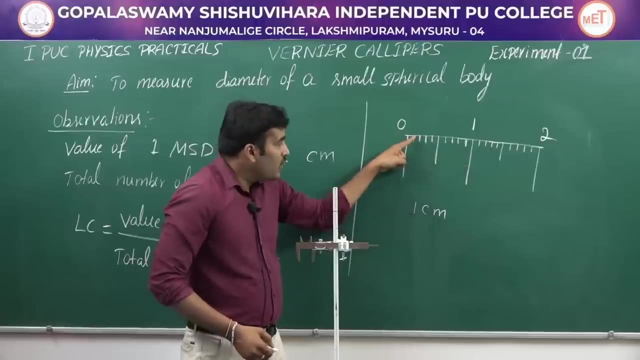 equal divisions. Therefore, here, if I want the value of one main scale division, So I said that from 0 to 1, from 0 to 1, the length is 1 centimeter and there are 10 equal divisions. So what is the value of this? 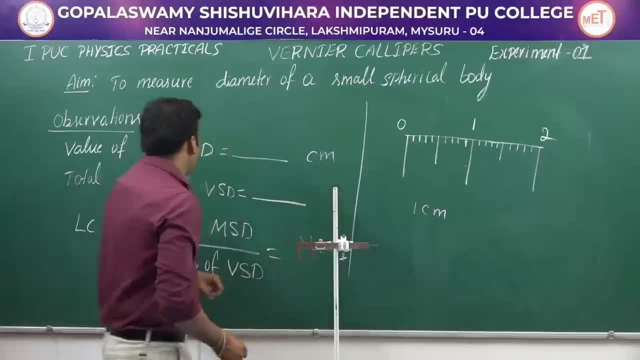 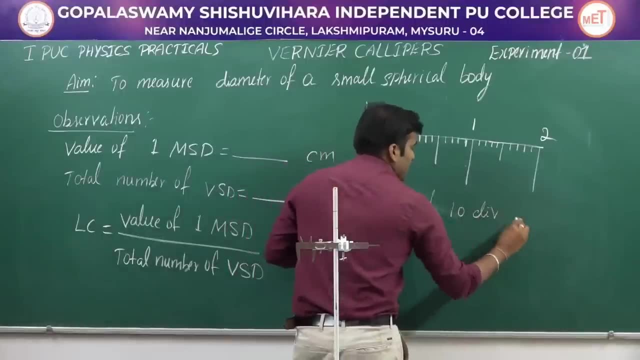 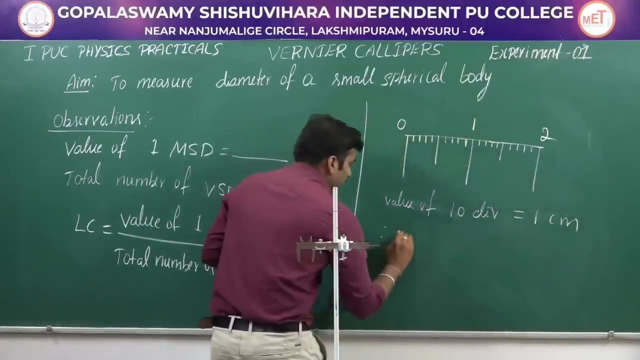 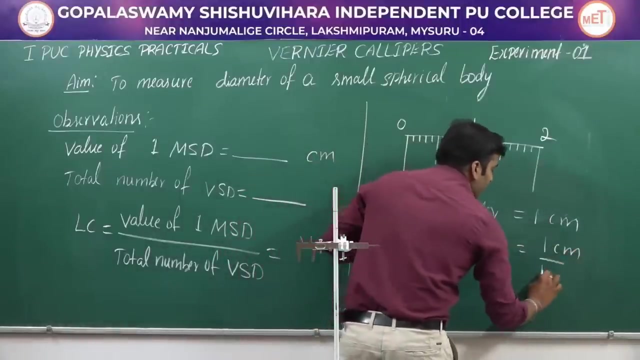 one division. What is the value of this one division? So that can be find like this: Value of 10 divisions is equal to value of 10 divisions is equal to 1 centimeter. therefore, value of 1 division will be 1 centimeter by 10.. That. 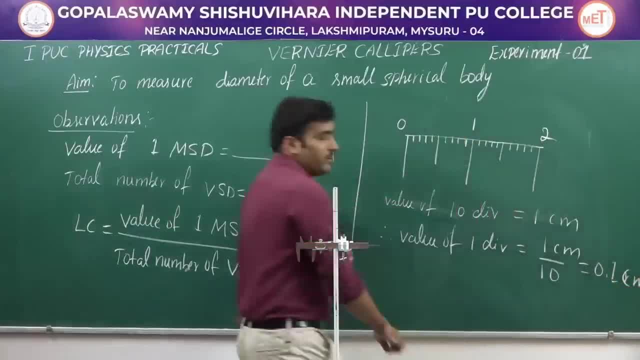 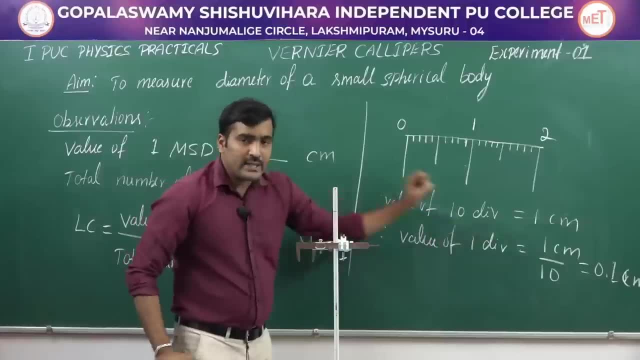 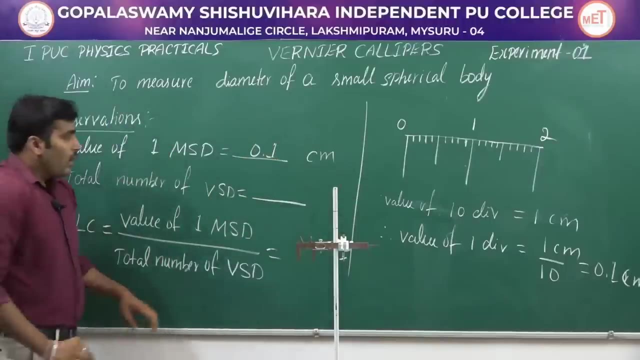 is equal to 0.1 centimeter. What is the value of 1 main scale division in the main scale of vernier, which is equal to 0.1 centimeter? So let us substitute this value of 1 main scale division is 0.1 centimeter. Next, 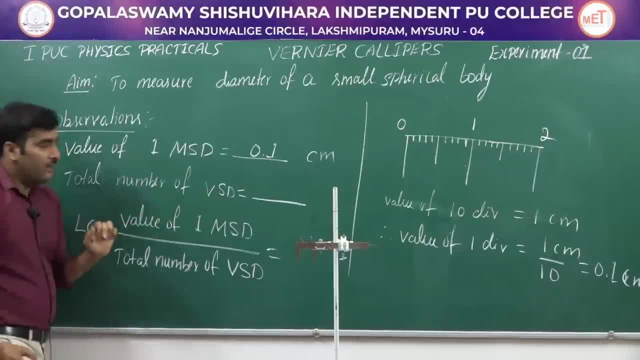 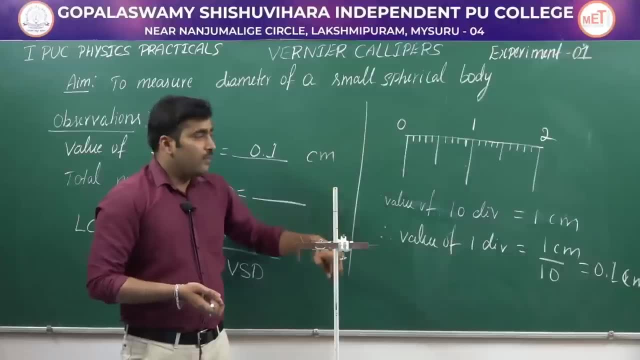 we have to find what is the total number of divisions on the vernier scale. So I said that there are two scales in your vernier calipers: One is a main scale and the other one is a vernier scale. So how many divisions are there in the 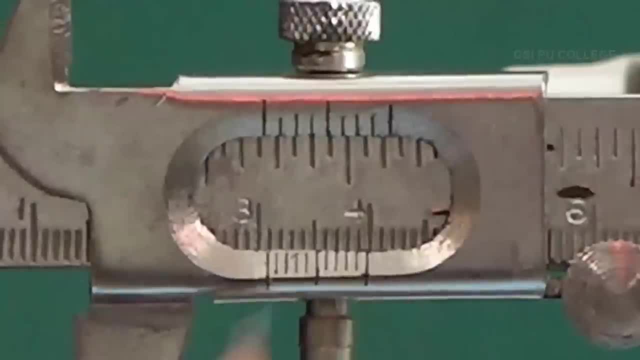 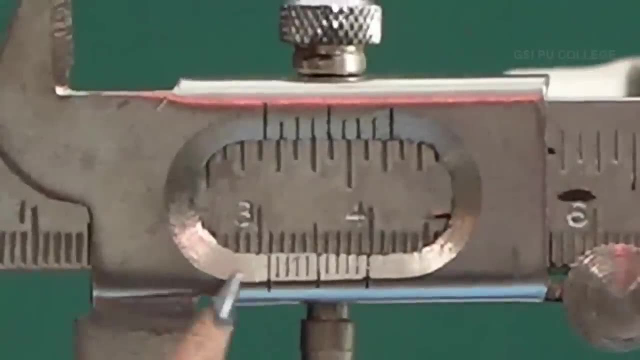 vernier scale That we have to find now. So this is your vernier scale, correct? So the first division is called zeroth division of the vernier. okay, This division, the longer line, is a zeroth division of your vernier. So, except this one, you need to count this. okay, How many divisions? 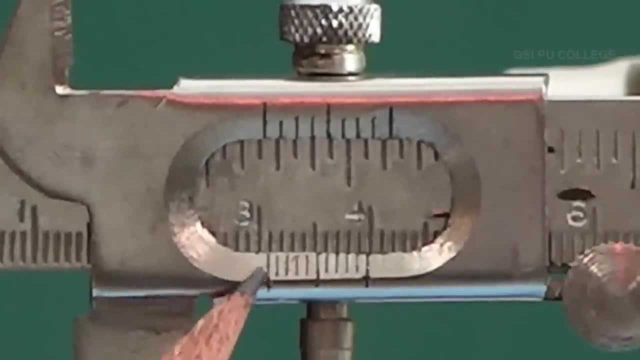 are there in this vernier scale, So leave this one. The first division is the zeroth division, and what are the remaining ones? You can find 10 divisions in this lower half. okay, There are 10 divisions in the vernier scale. okay, There are totally 10 divisions. Actually, there are 11. 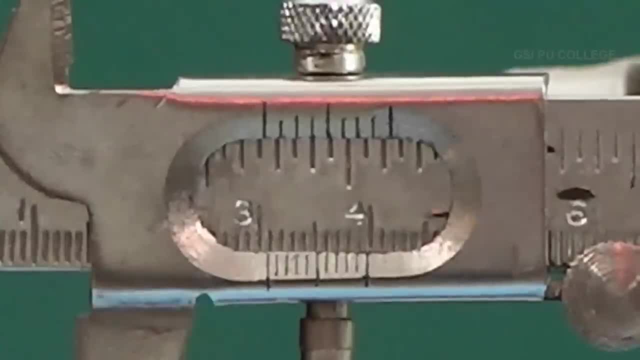 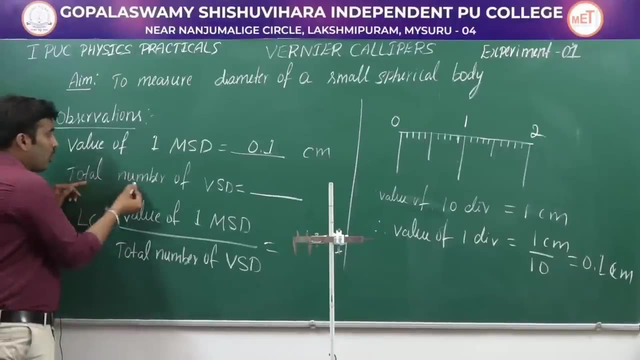 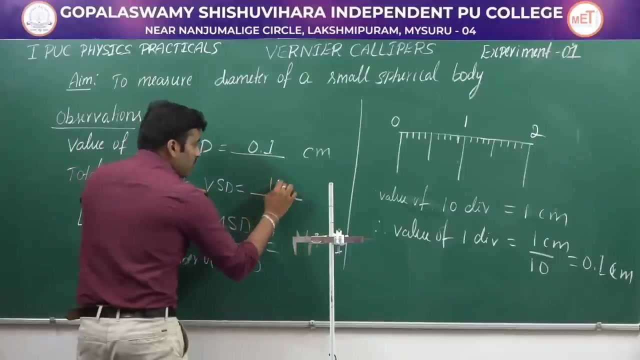 divisions. The first division is considered as a zeroth division. That is why the remaining one will be 10.. So let us substitute the total number of VST. VST means vernier scale divisions, So we have counted that It is equal to 10.. So there are 10 divisions in. 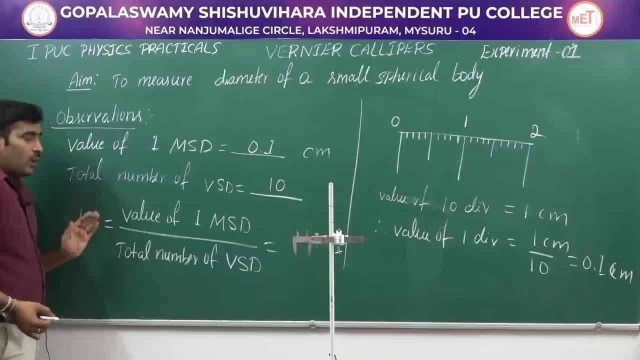 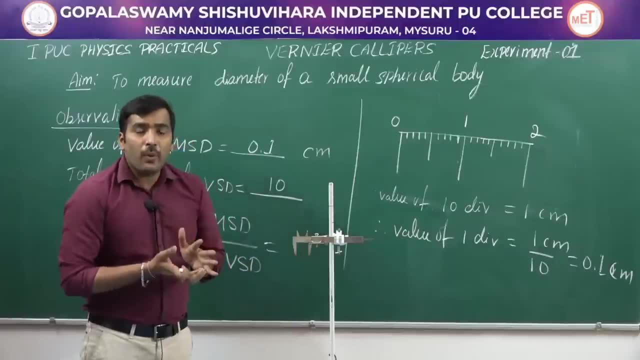 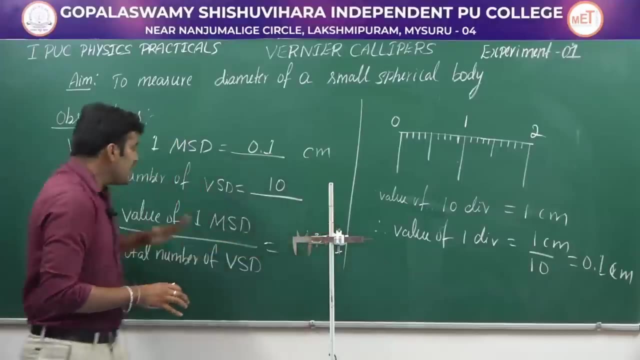 the vernier scale. Next, we need to find the least count. LC refers to least count. What do you mean by a least count? Least count is the lowest possible value that can be measured by any instrument. Okay, For the vernier calipers, the least count is found using this formula: okay, Least count is: 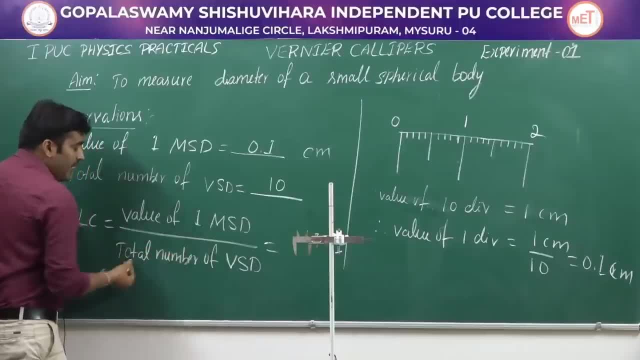 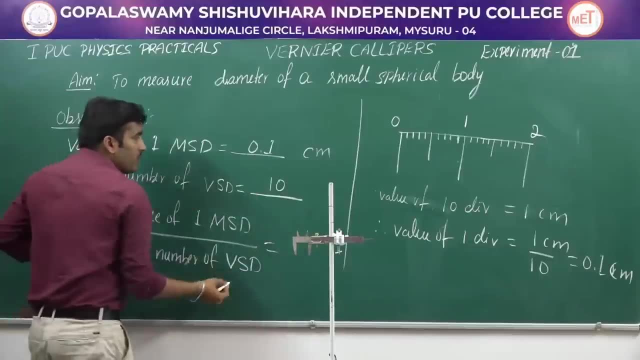 equal to value of 1 MSD divided by total number of VST. okay, So we have values of 1 MSD and total number of VSTs here. Let us substitute that The value of 1 MSD is 0.1 centimeter. Therefore, 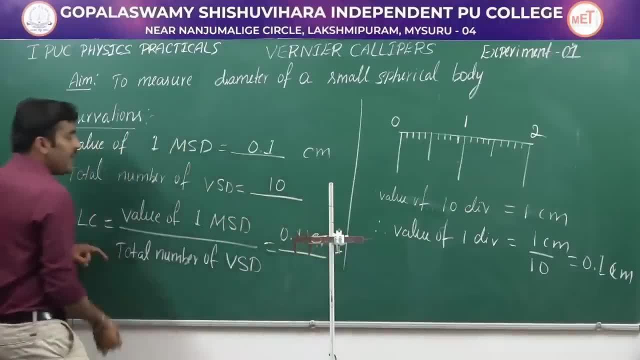 this is 0.1 centimeter divided by total number of VST is 10.. Therefore, this is divided by total number of VSTs. So this is 0.1 centimeter divided by total number of VSTs. So 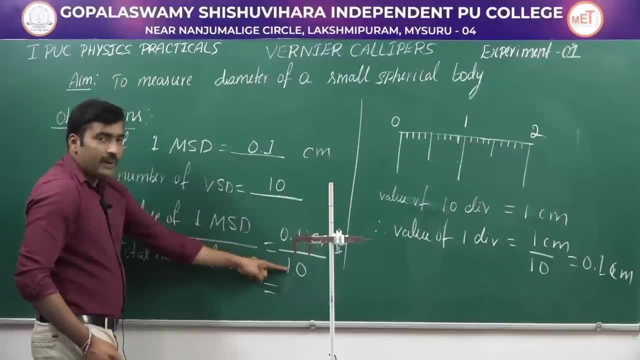 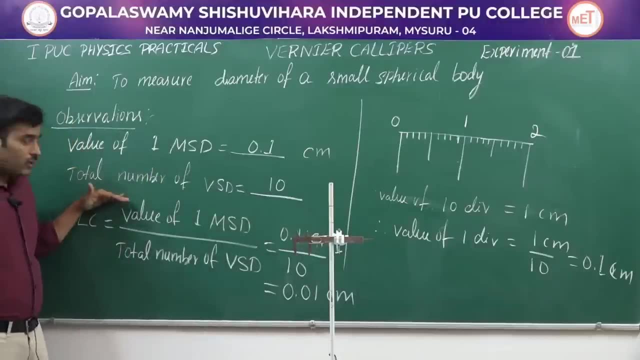 this is 0.1 centimeter divided by 10.. So let us divide this 0.1 centimeter by 10.. This will be equal to 0.01 centimeter. Therefore, the least count of the vernier calipers is equal to 0.01. 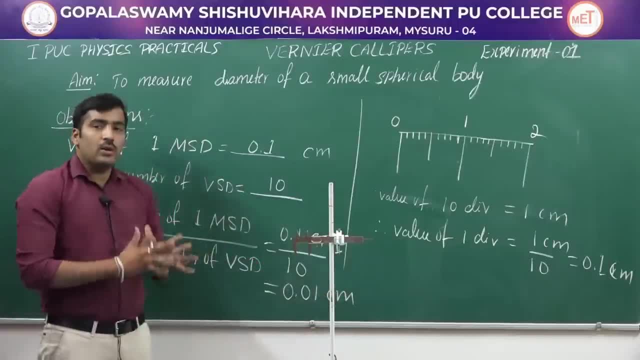 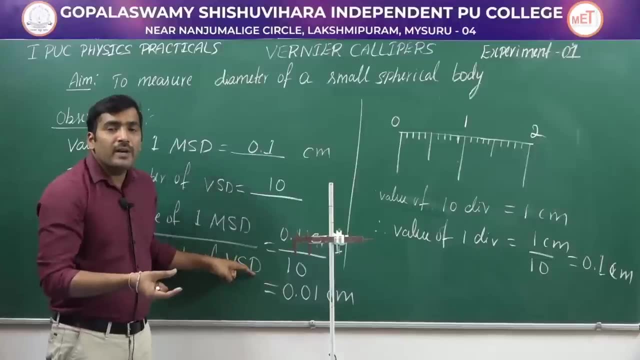 centimeter. So you know what is least count. A least count is the lowest possible measurement that can be done by an instrument. So, by using vernier calipers, what is the least value you can measure? The value is 0.01 centimeter. Okay, Yes. 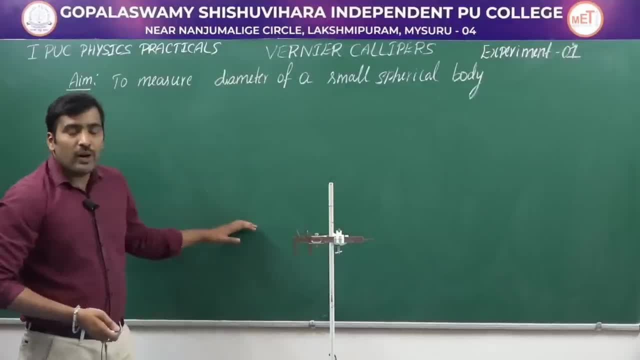 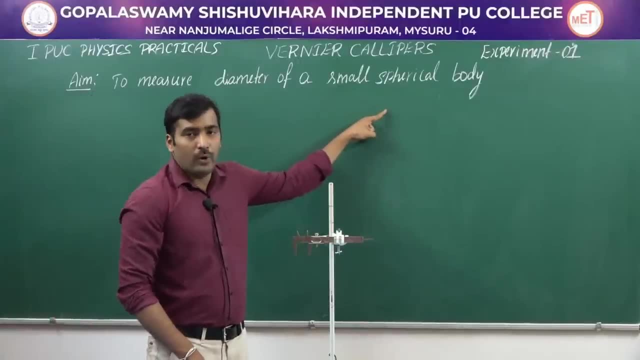 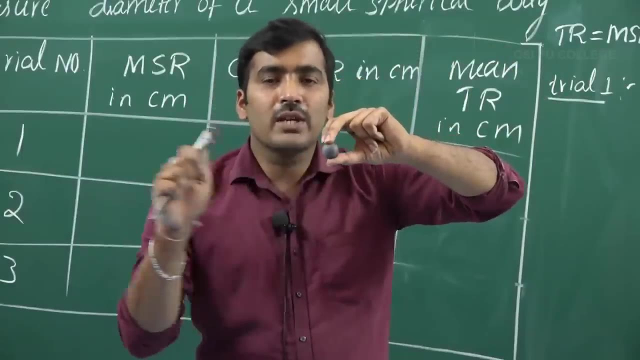 So what is the aim of our experiment here By using vernier calipers? what we need to measure now is to measure the diameter of a small spherical body. okay, See, this is the spherical bob, and we need to find the diameter of this spherical bob using the vernier calipers. So I said that. 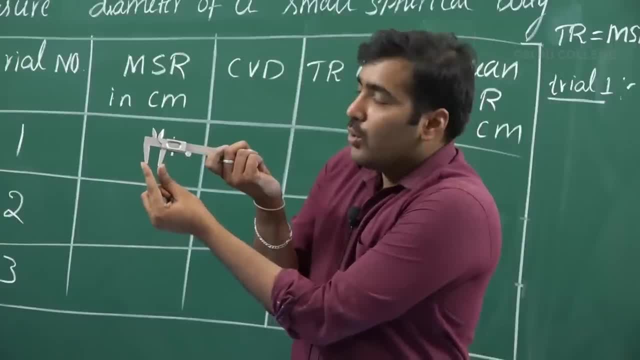 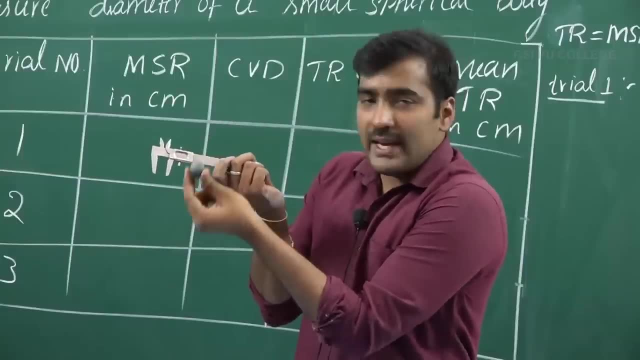 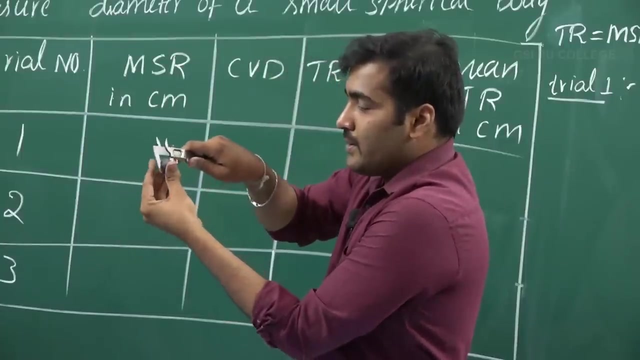 these are the pair of lower jaws where we have to place the object in order to find the diameter of the spherical body. So we need to find the diameter of the spherical body, So we need to place this between the lower jaws of the vernier calipers. So let us place that. So this is how. 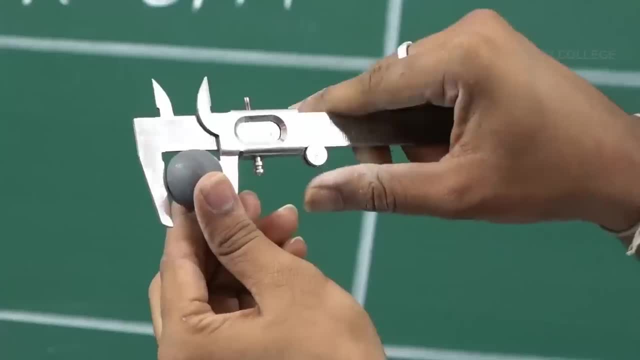 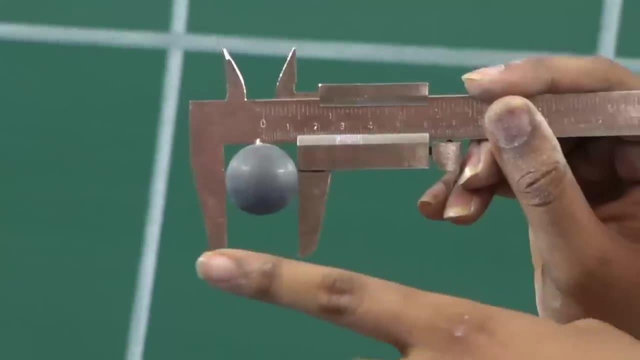 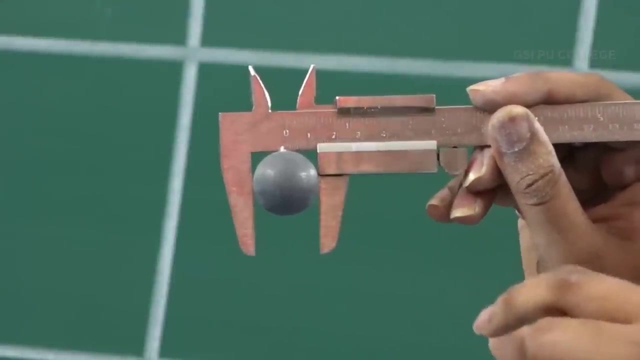 you have to place it and you just move this one. okay, So you can scroll the vernier scale towards this bob, and so the object must be placed between the lower jaws of the vernier calipers and you can slide the vernier towards the bob so that it can fit into the jaws properly. okay, So this is the 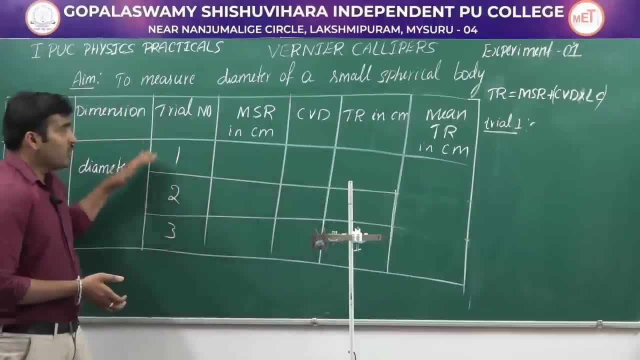 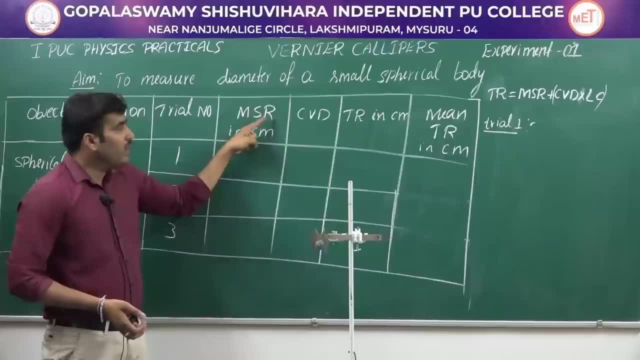 diameter of the spherical body. So this is your tabular column. okay, So here you can find MSR. What is this MSR? Main scale reading. okay, This is main scale reading. I already told you that there are two scales in your vernier calipers, So you need to find the two readings here. okay, One is: 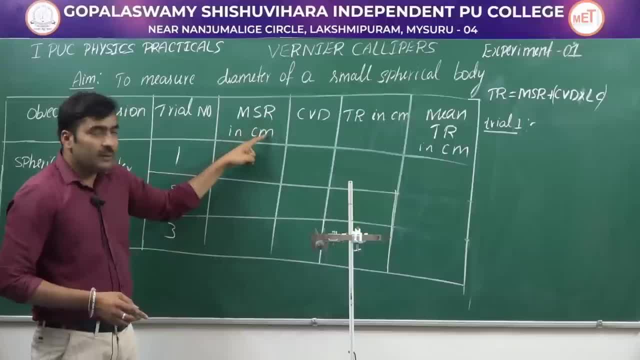 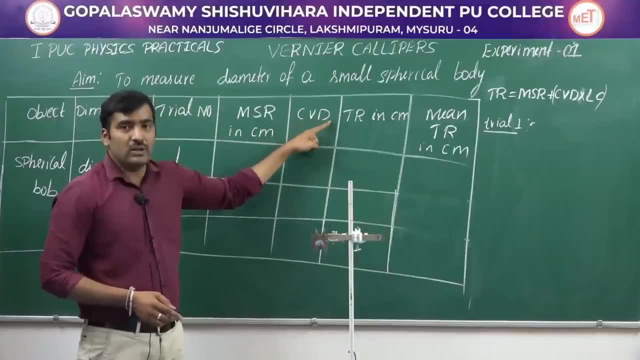 a main scale reading. MSR is main scale reading, This is in centimeter, and this one is CVD. CVD refers to coincided vernier division. okay, So this is the main scale reading. So this is the coincided vernier division. So this is just a number, okay, So here you will not find any. 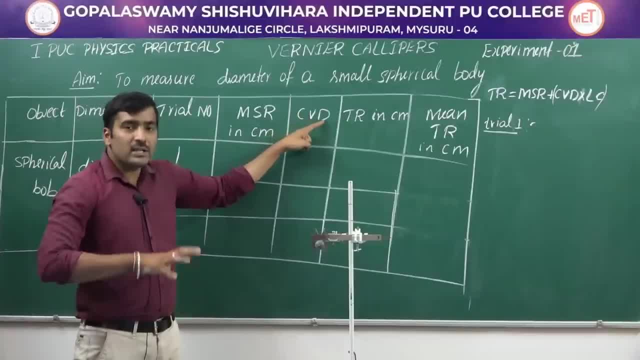 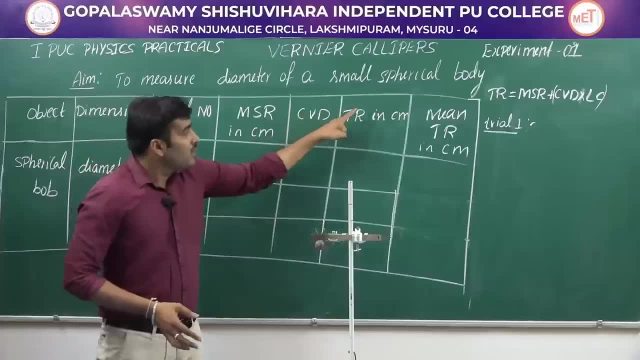 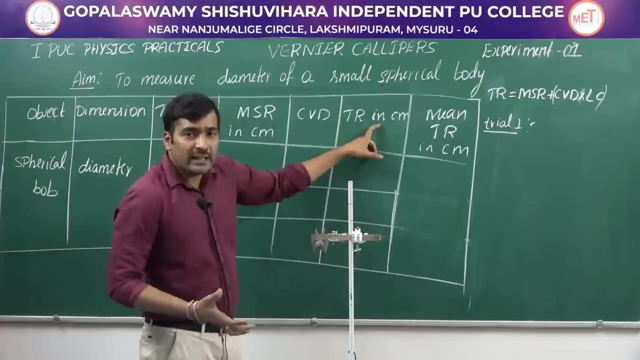 centimeter or meter. likewise, because this CVD is just a number, It is not a measurement, Let us find the value of main scale reading first. Then let us find the CVD, and this is TR. TR refers to total reading. okay, TR is total reading. How do you find the TR? This is a formula, See TR is. 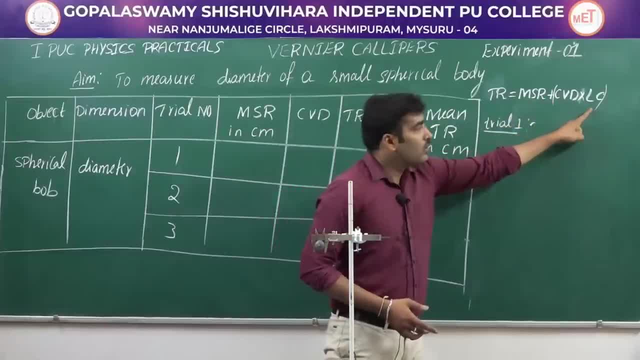 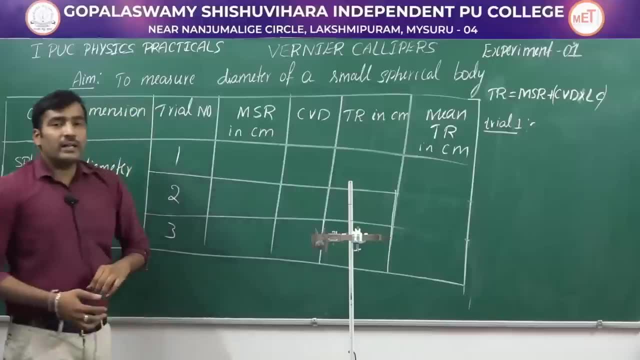 MSR plus CVD, CVD into LC. LC is least count. okay, So this is the formula for finding the total reading. So you have to take the three readings, okay? For the same object, the same dimension, that is, diameter. 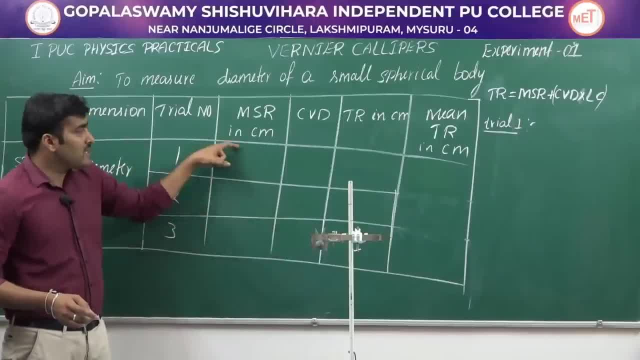 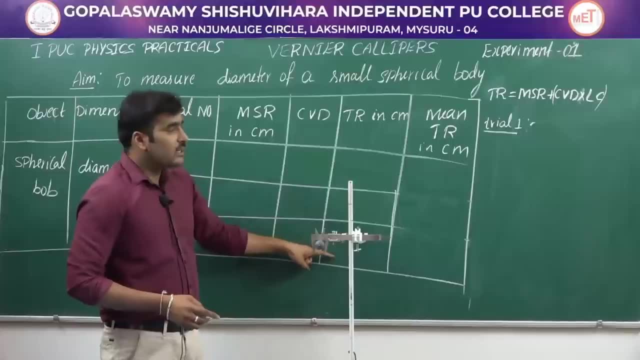 is to be find three times. okay, You have to make three trials- MSR and CVD, MSR and CVD, and MSR and CVD likewise, And you find TR for all these three readings. Then you should take the mean value of. 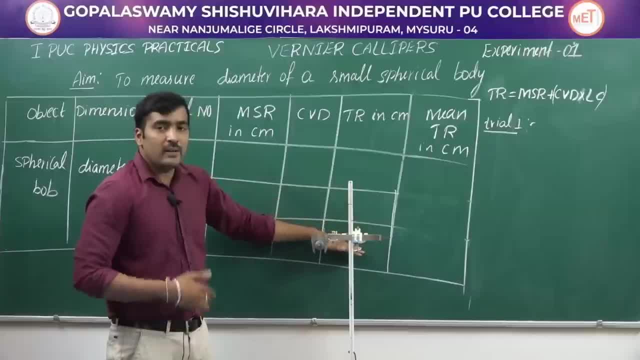 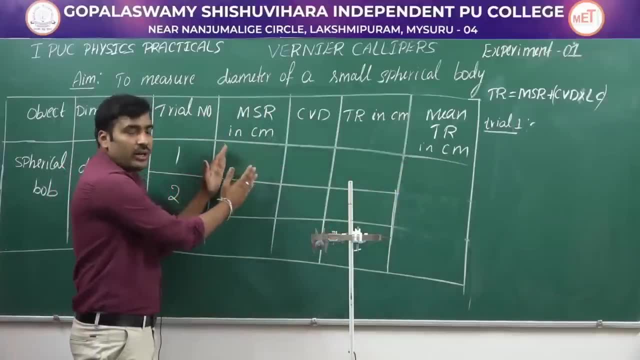 it okay. Mean value is sum of these three readings. So you have to find the TR for all these three measurements divided by number of measurements. So then we can find this TR. okay, First let us find this MSR. okay, How do you find the MSR? That is main scale reading. So how do we find the main? 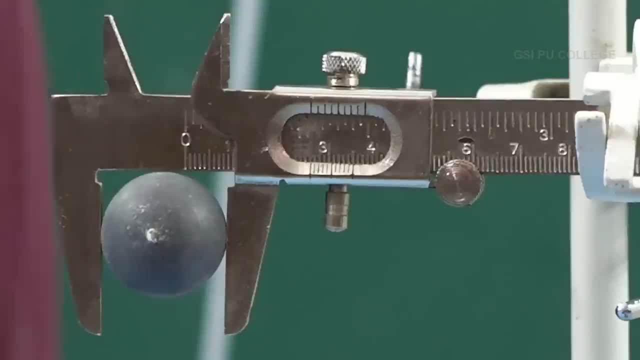 scale reading first. So for the main scale reading first you need to observe the zeroth division of the zeroth division of the Vernier scale. okay, So I said that this one is the zeroth division. okay, This is the zeroth division. 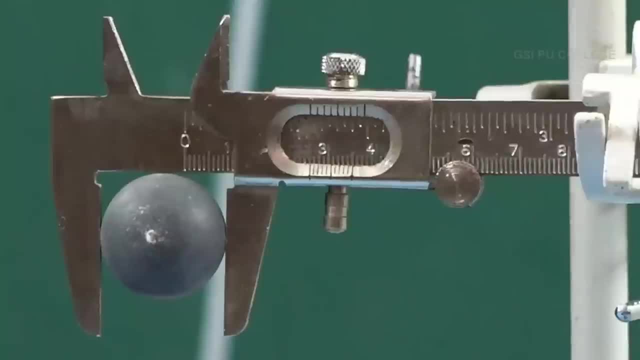 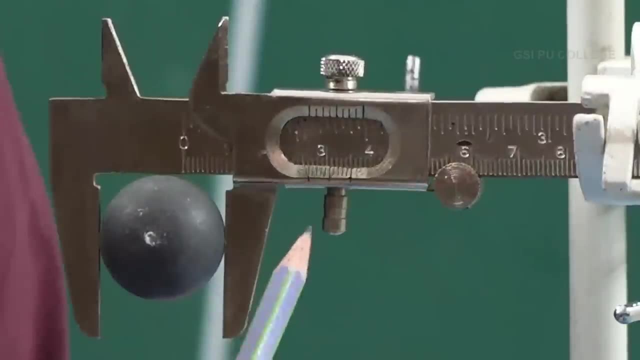 So if you observe the zeroth division of the Vernier scale, it is in between the two divisions of the main scale, correct? So which are those divisions? So the zeroth division of the Vernier scale is in between 2.6 and 2.7 of the main scale. okay, Therefore you should take the least one as. 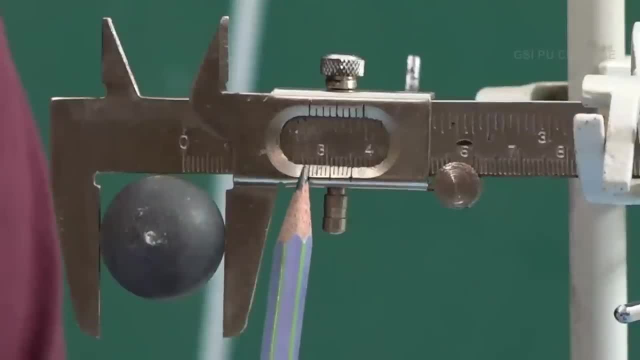 the main scale reading. okay, The zeroth division of the Vernier is in between the two divisions of the main scale, that is, 2.6 and 2.7.. Therefore, the least division is 2.6 centimeter. 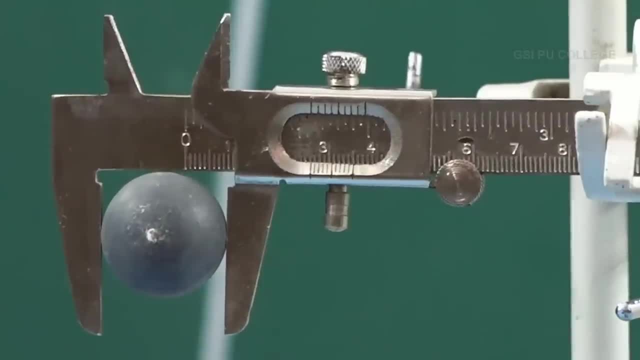 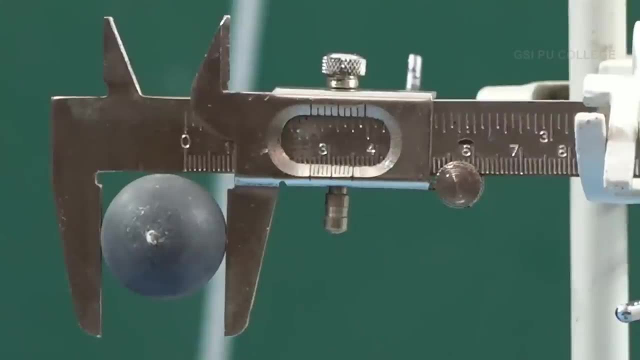 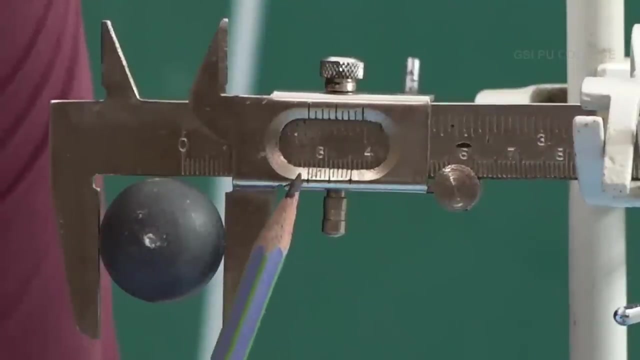 So you should consider the 2.6 centimeter as MSR. Next we need to find the CVD here. CVD is coincided Vernier division. How do you find the coincided Vernier division here? See the zeroth. 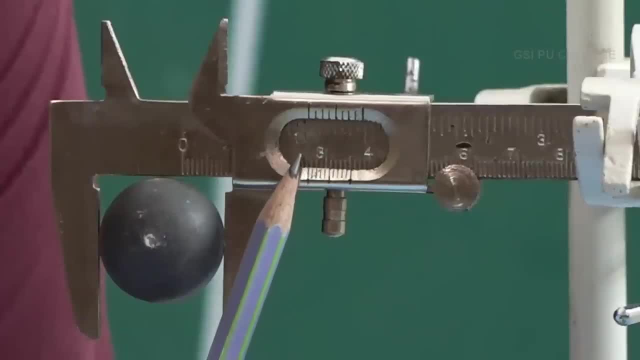 division is in between the two divisions of the main scale. The first division is also in between the two divisions of the main scale, But if you observe the second division properly, the second division is exactly coincided with the one of the division of the main scale. okay, So the second division in the Vernier. how do you count this? This is the 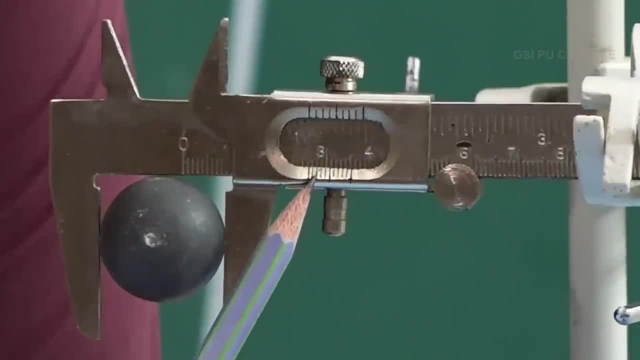 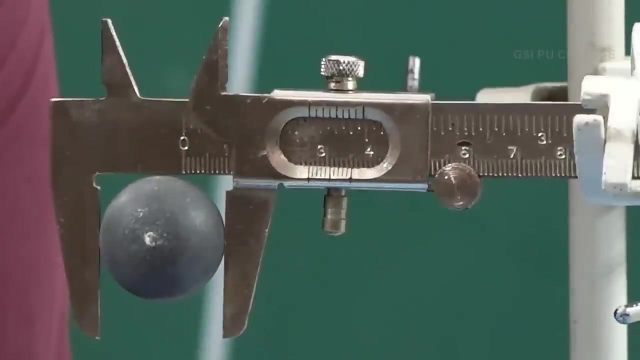 zeroth division. correct. The next division is first. The next division is second division. So the second division of the Vernier scale is exactly coincided with one of the division of the main scale. Therefore the second division, or two, is considered as coincided Vernier division. So you will be considering the second. 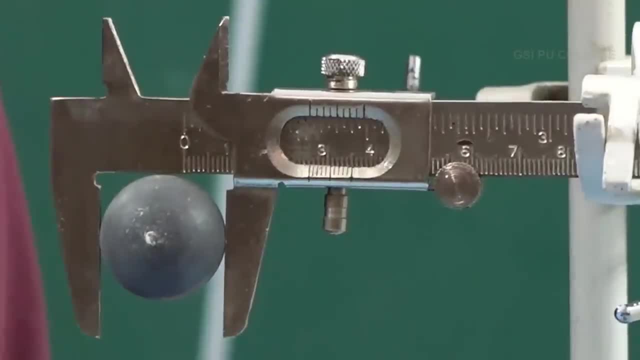 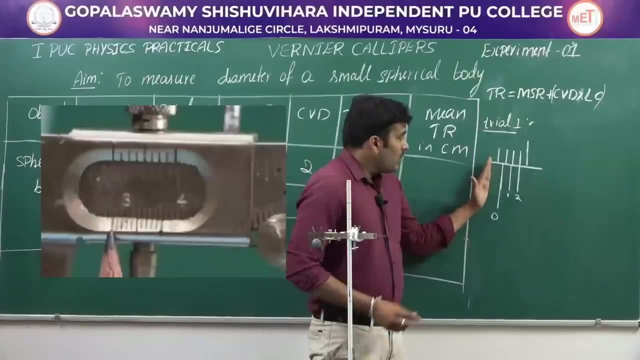 division of the Vernier to be the coincided Vernier division, because it is exactly coincided with the one of the division of the main scale. You can observe here: This is the zeroth division. okay, This is the zeroth division of the. 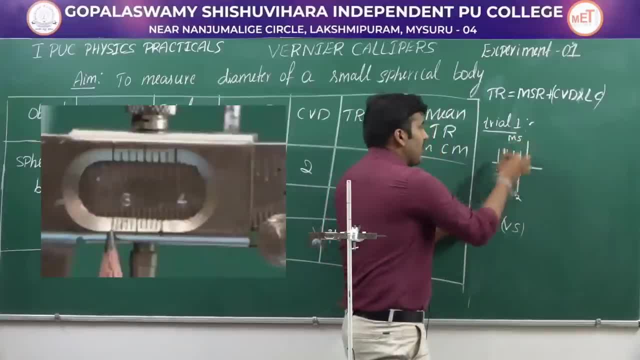 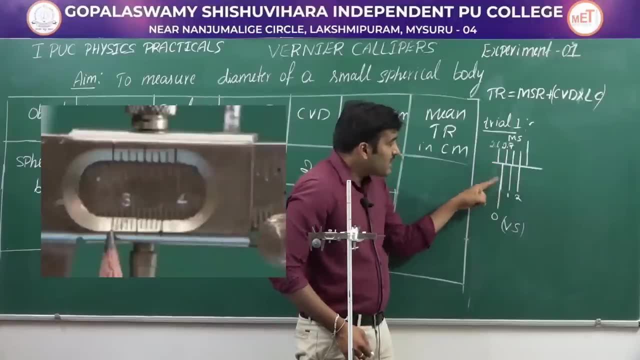 MetaOS. So if I conjugate these two divisions you can see that the zeroth division of the main scale- vernier scale- this is vernier scale and this one is a main scale. so in the main scale this is the 2.6 and this is 2.7. so the zeroth division of the vernier scale is lying between 2.6 and 2.7. 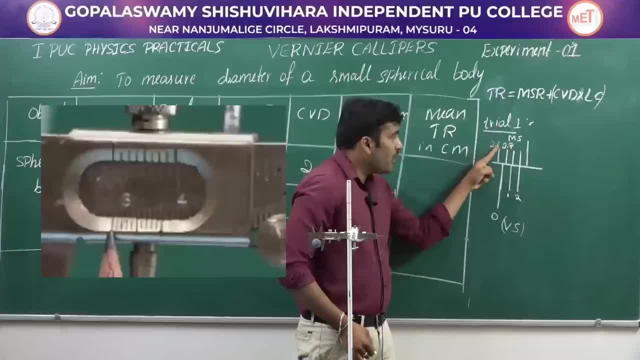 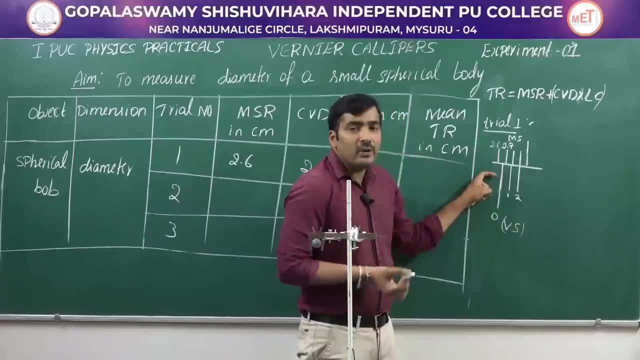 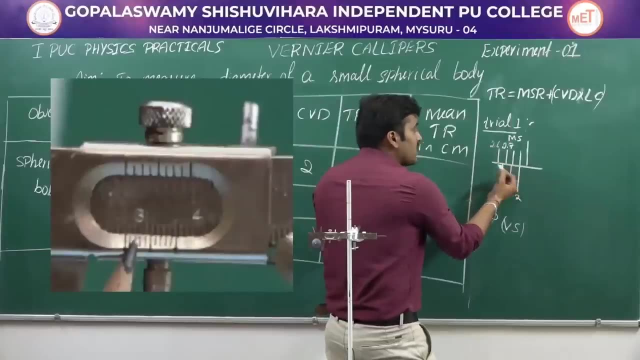 centimeter of the main scale. that is why the least division is 2.6. that is why we have written 2.6 centimeter as msr. next, how do you find the coincided vernier division? see, this division is in between the two divisions of the main scale and this division is also very near to this. 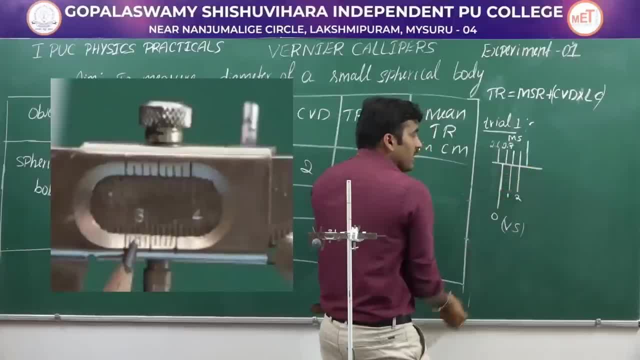 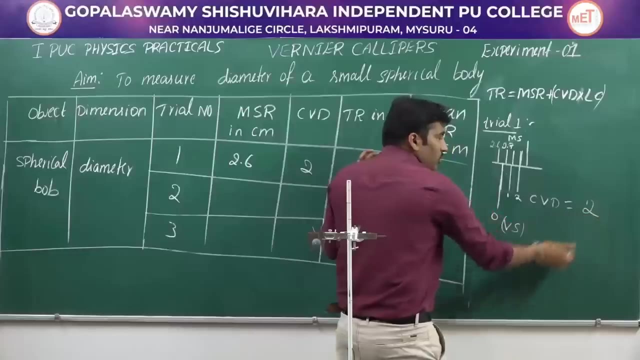 division. but the second division of the vernier scale is exactly coincided with this division of the main scale. that is why this division is considered as coincided vernier division. so coincided vernier division here is: cvd is equal to 2. so that is why we have written this cvd as 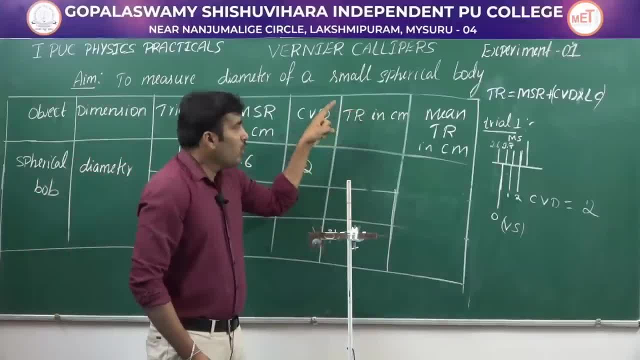 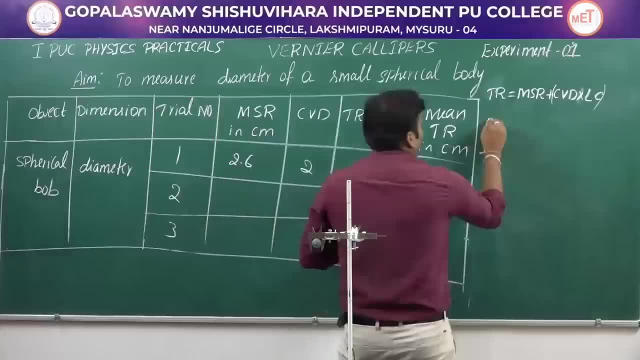 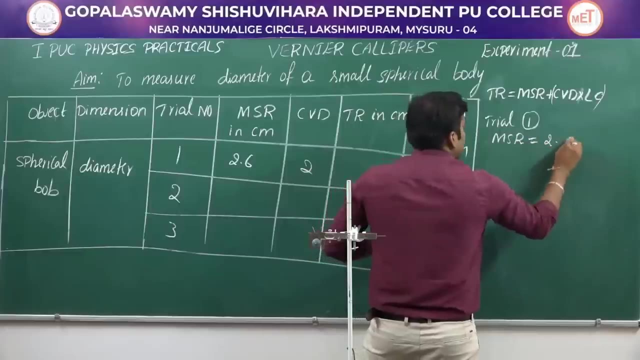 2 here. okay, next let us find this tr. how do you calculate this tr? we have a formula: tr is equal to msr plus cvd into lc. let us find out the value of tr for trial number one. main scale reading is equal to 2.6 centimeter, cvd is equal to 2 and lc is equal to 0.01 centimeter. 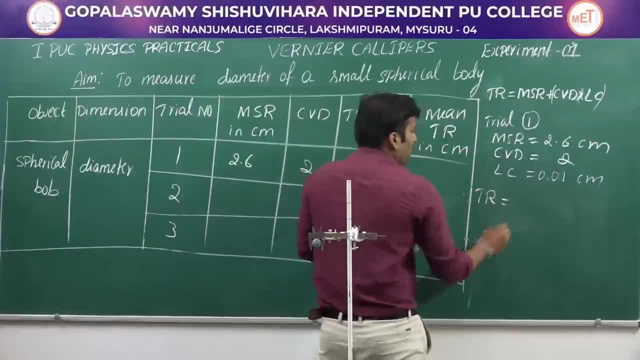 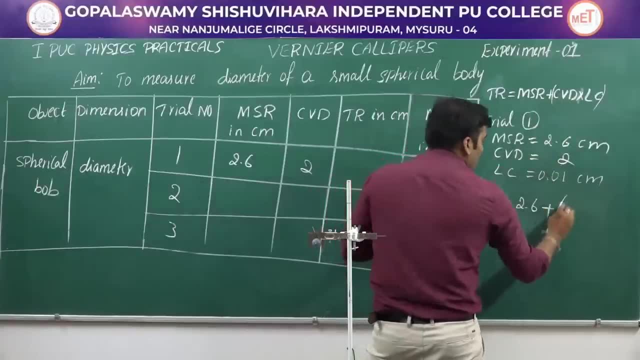 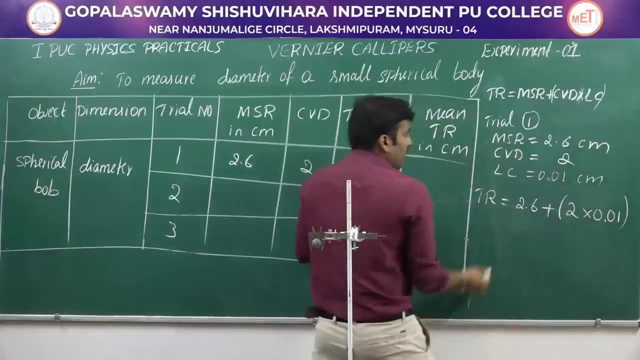 so let us substitute these values here. so tr is equal to msr is 2.6. let us write that 2.6 and lc is equal to 0.01 centimeter, so let us substitute these values here. 2.6 plus CVD is 2.. This is 2 into LC is 0.01 centimeter. Therefore, this is 0.01 centimeter. 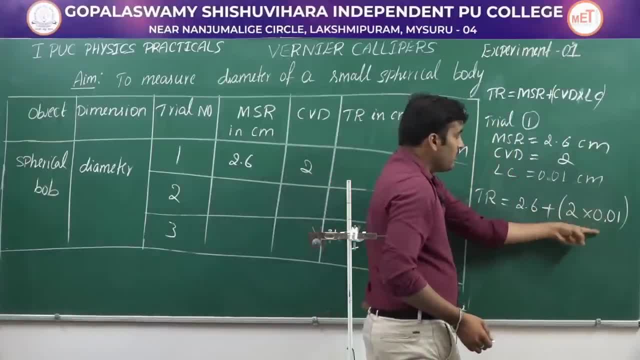 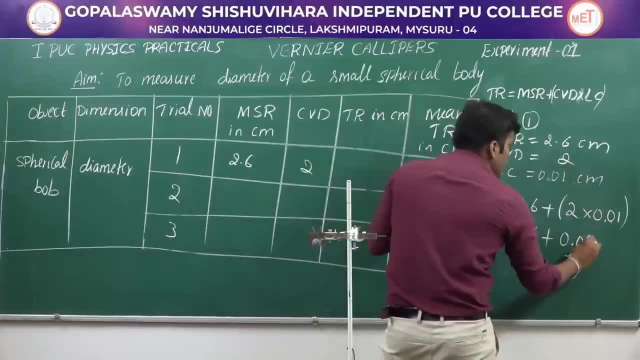 First you should multiply these two, and then this term should be added to this one, So 2.6- keep that as it is- 2 into 0.01 is 0.02.. Then you should add these two: 2.6 plus 0.02 is 2.62. 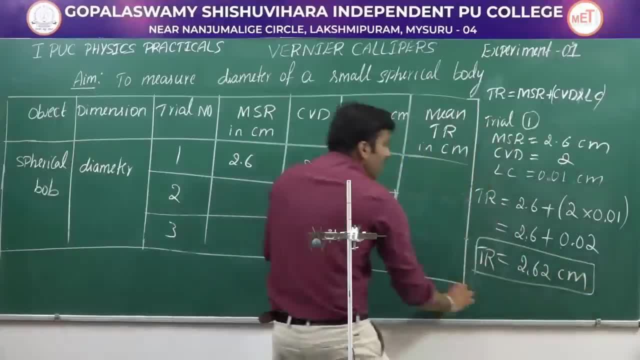 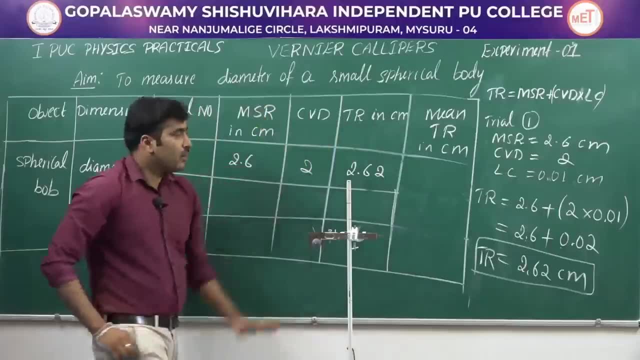 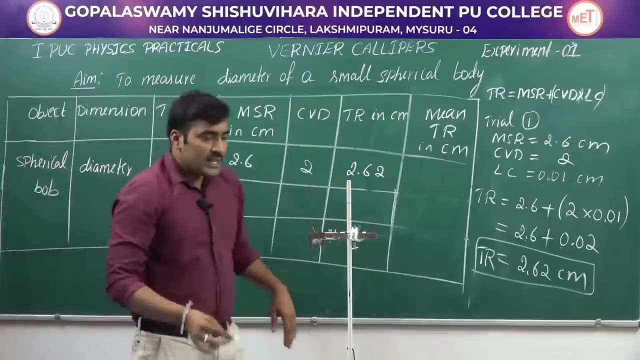 centimeter. Therefore, the total reading will be 2.62 centimeter. Let us write that this is equal to 2.62 centimeter. Now we need to find the diameter of the same spherical body by changing the position For the second trial. let us change the position of this spherical body. 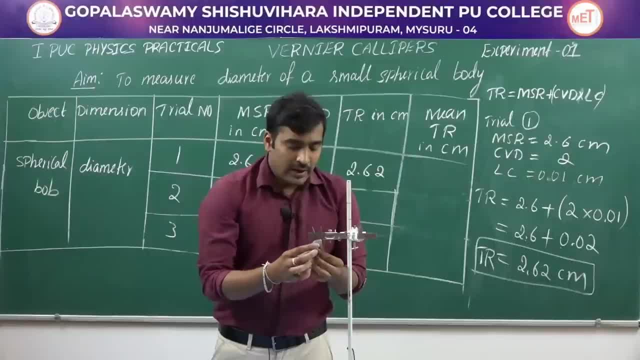 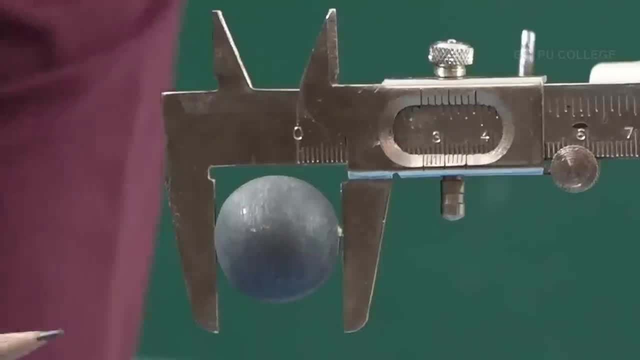 slightly. I am just changing the position and again I have to place the object in the same way. Now I have slightly changed the position of the bar and now we are taking the second trial. Let us find out the values of main scale reading and CVD So you may observe the 0th division. 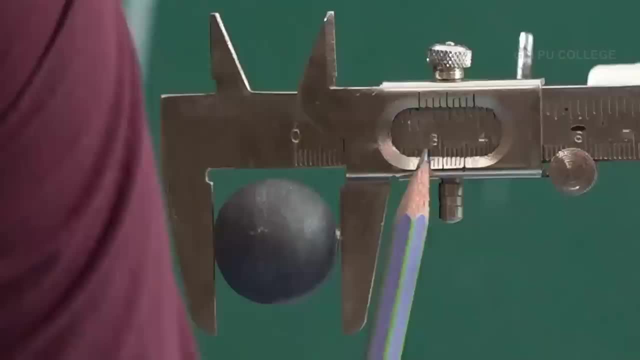 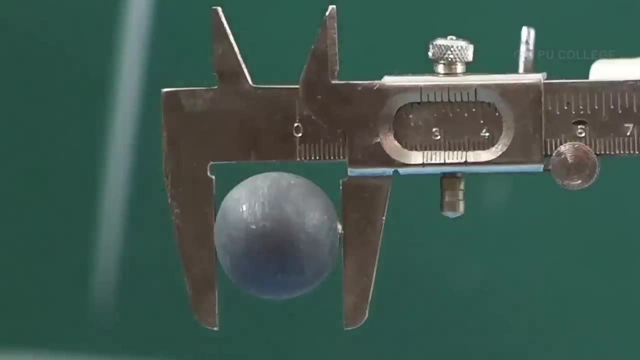 of the vernier is now again lying between 2.6 and 2.7 centimeter of main scale. Therefore, we can consider the main scale reading as 2.6.. Now we should observe the coincided vernier division, that is, CVD. 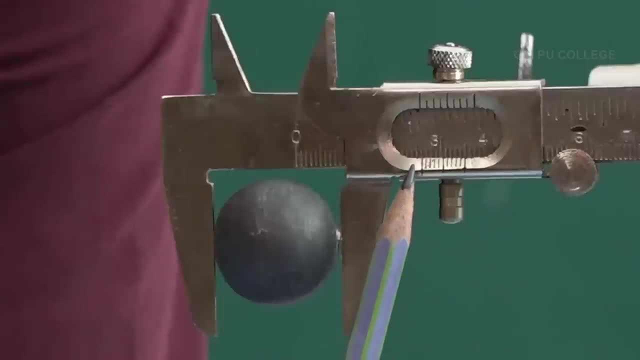 So first division, that is, the 0th division, is in between the two lines of the main scale. The next division, the first division. Now the first division is coincided exactly with the main scale division. That is why in this case the CVD is considered as 1.. You can observe here: 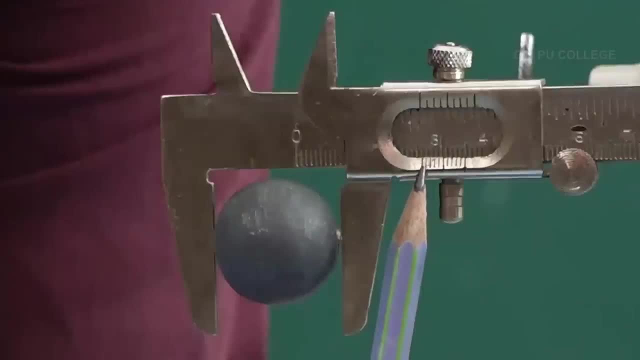 this is the 0th division. 0th division is in between the two lines, but the very next division is coincided with the division of the 0th division. So the 0th division is in between the two lines. 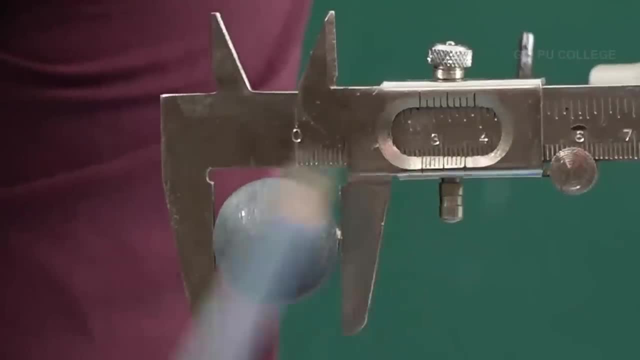 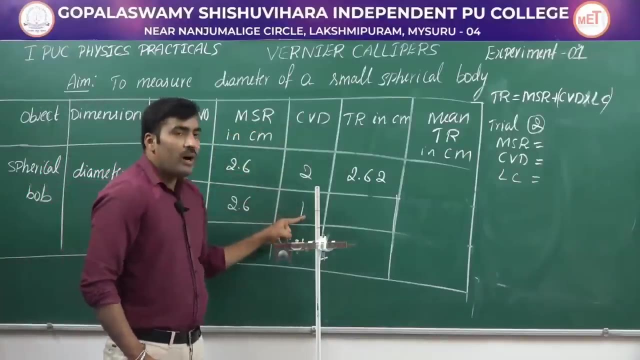 That is why the CVD coincided vernier division here becomes 1.. For the second trial, the main scale reading is turned out to be 2.6 and the CVD is equal to 1.. Let us find out the total reading now. 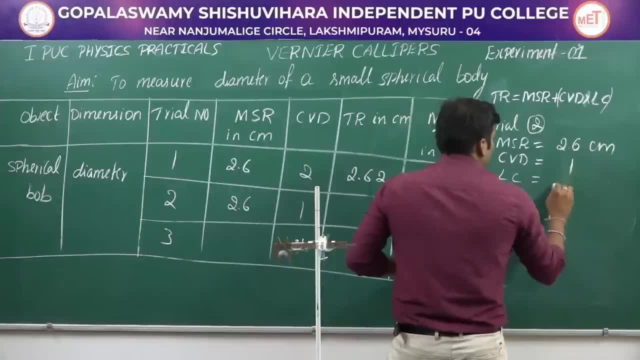 MSR is 2.6 centimeter, CVD is 1.. LC is 0.01 centimeter. So let us find out the TR Main scale reading is 2.6.. This is 2.6 plus CVD is 1 into least count. 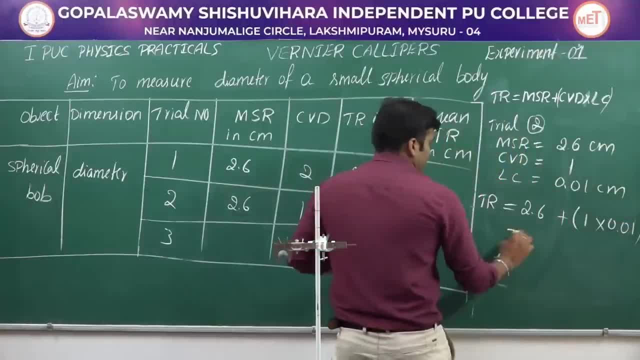 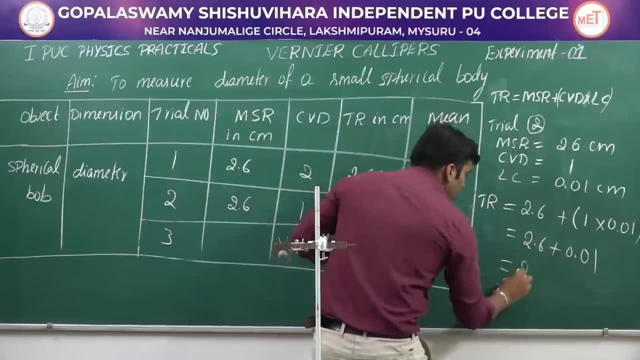 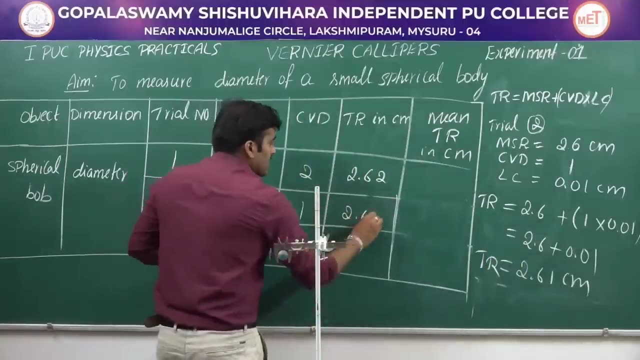 LC is same 0.01 centimeter. Now 2.6 plus 1 into 0.01 is 0.01.. Now let us add these two, This will be 2.61 centimeter. Therefore, total reading for the second trial will be 2.61. 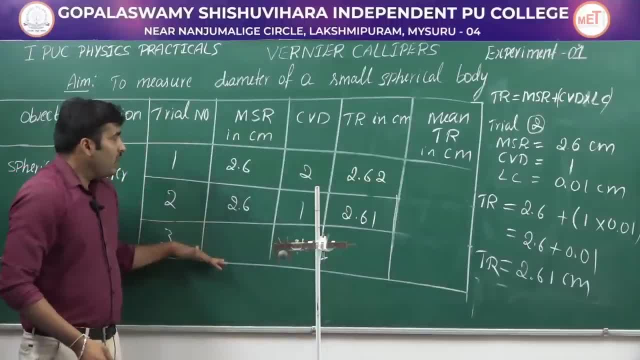 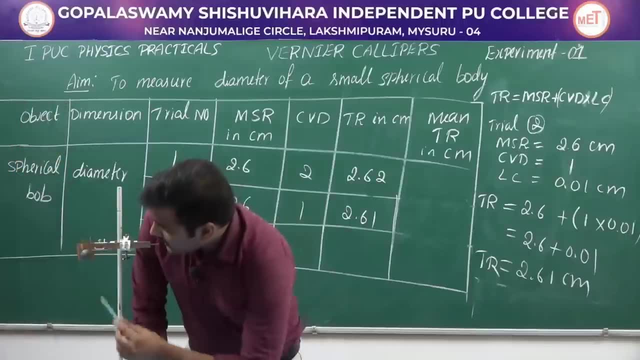 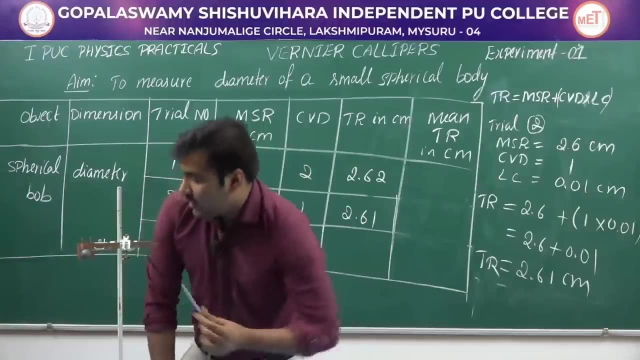 centimeter. Now let us find out the last trial. For the third trial, again, let us find out the main scale reading and coincided vernier division. So for the third trial, main scale reading is 2.6 and the coincided vernier division is equal to 5. So let us write that: 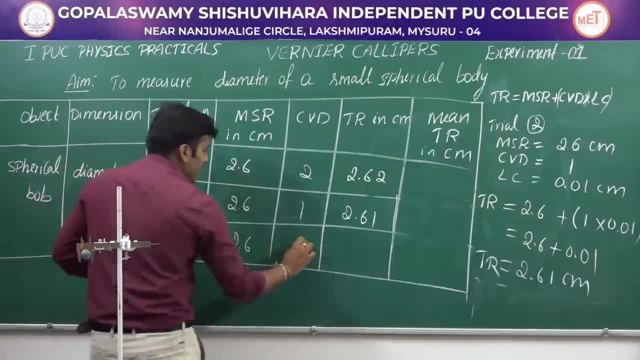 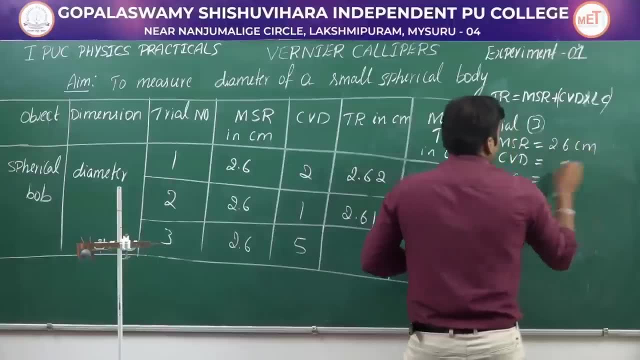 2.6 and the CVD is equal to 5.. Let us find out the total reading. So for the third trial, main scale reading is 2.6 centimeter coincided vernier division is 5 and least count is same. 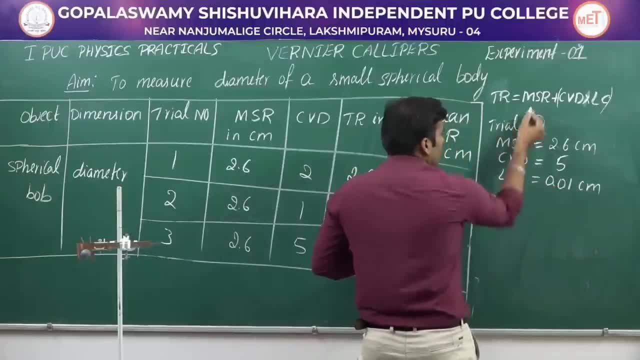 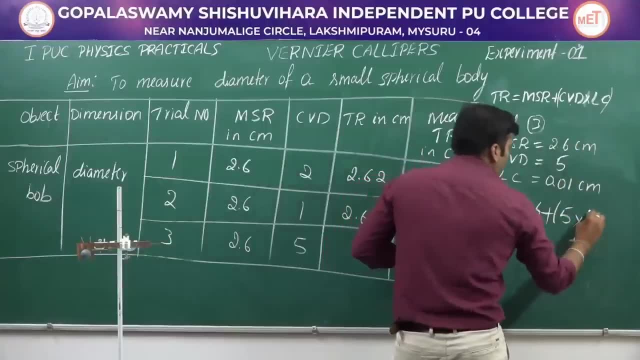 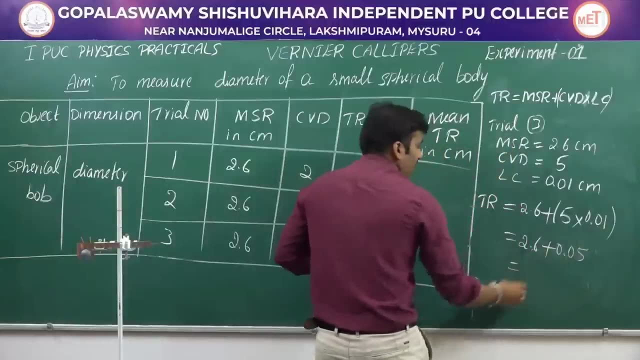 0.01 centimeter. Let us substitute the values: MSR is 2.6 plus CVD is equal to 5 into least count is 0.01.. Next, 2.6 plus 5 into 0.01 is 0.05, and if you add these two you will get 2.65 centimeter. 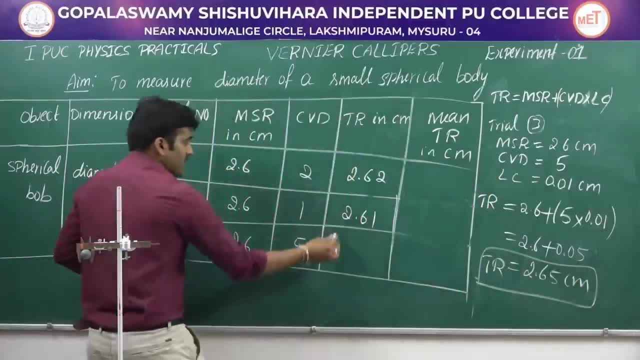 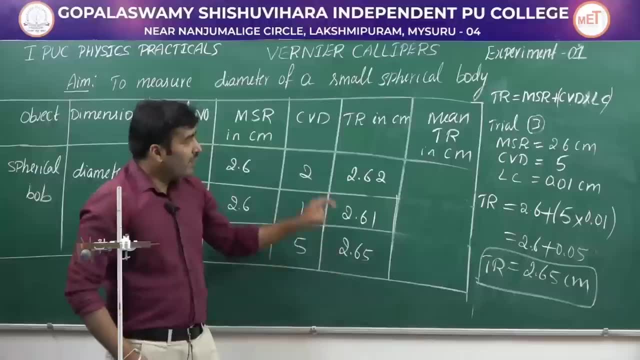 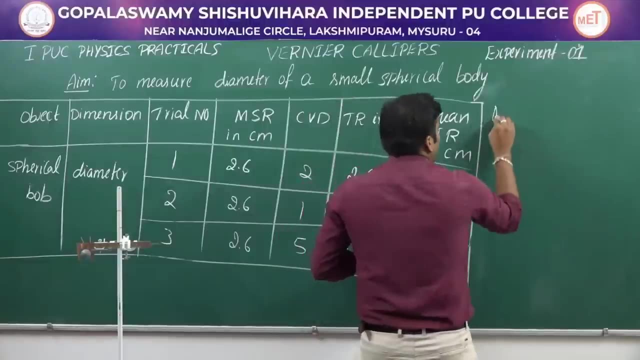 Therefore, the third trial is 2.65 centimeter. Let me substitute this: This is 2.65.. Next, in the last column, we need to find the mean value or the average of these three. Let us find out that. So how do we find this? mean TR, Mean TR. so we need to add these three trials. 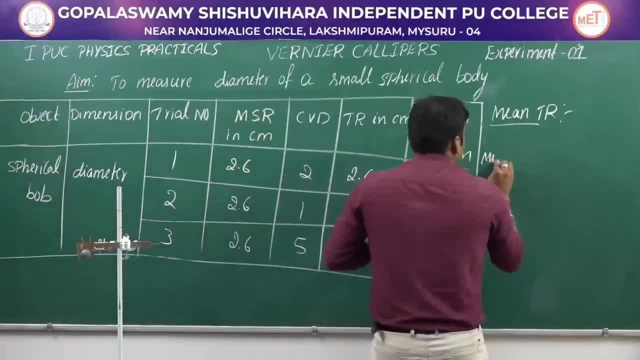 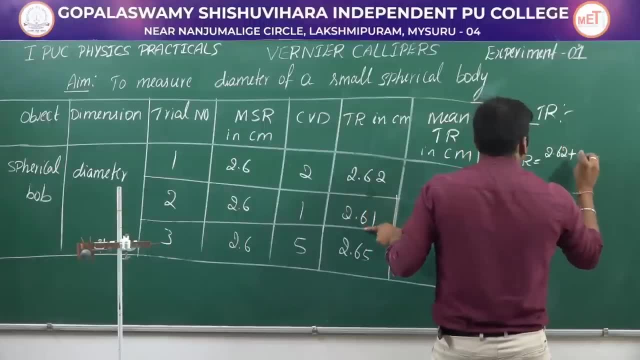 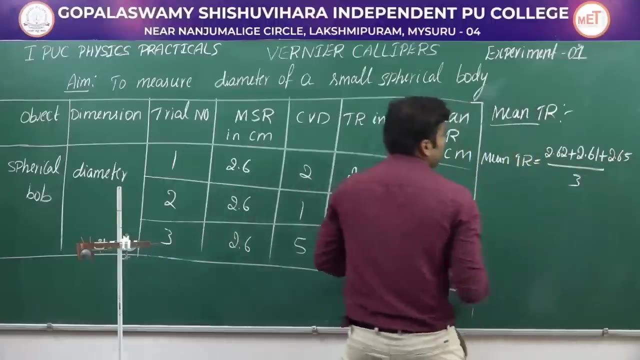 and divide it by 3.. So mean TR is equal to 2.62 plus 2.61 plus 2.65.. 4 divided by 3. The value of mean TR is now found to be 2.626.. But according to the rule, 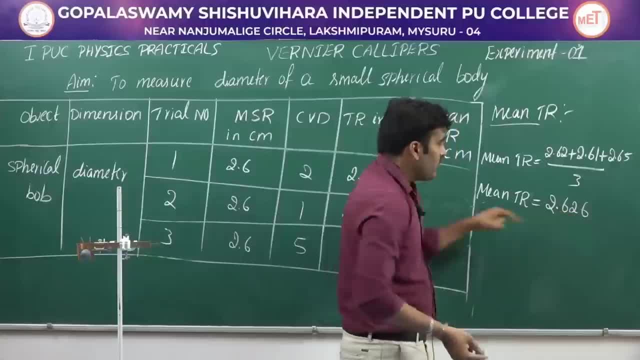 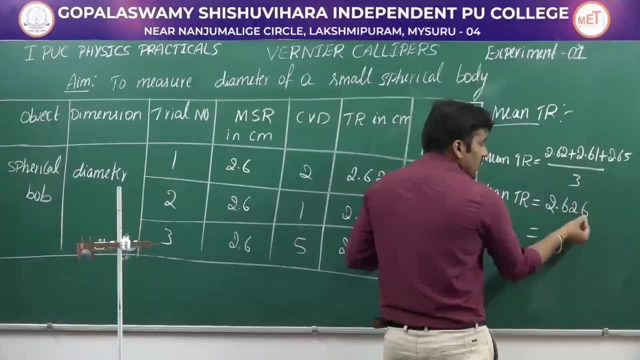 of significant figures, we need to keep up to the second decimal place. So let us round off this. This is 6.. So if the value that has to be rounded off is more than 5, then the preceding digit must be increased by 1.. Therefore, this will be 2.63. 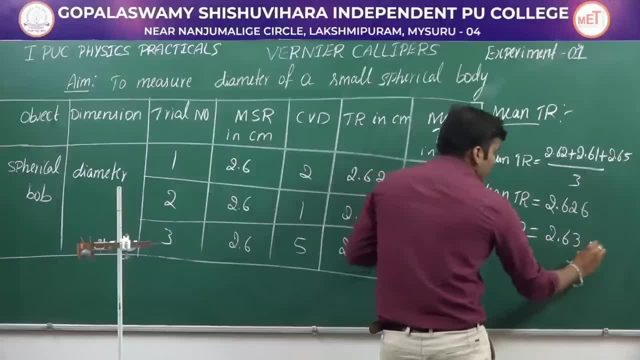 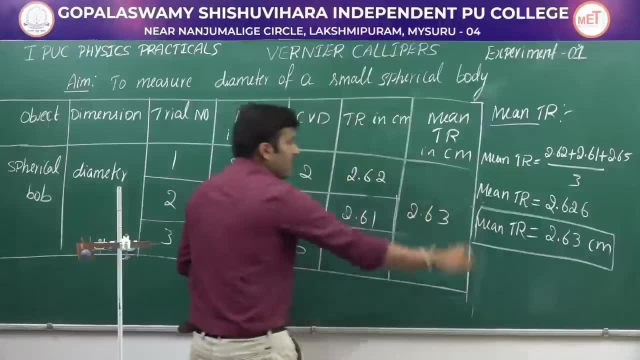 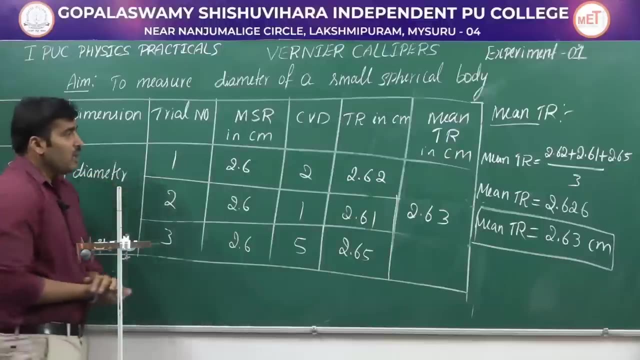 Therefore, the mean TR, the value of mean TR, is equal to 2.63 centimeter. Then you substitute here you will get 2.63.. So this is how you can find the diameter of the spherical body using the vernier calipers. Now let us write the result, the final result. 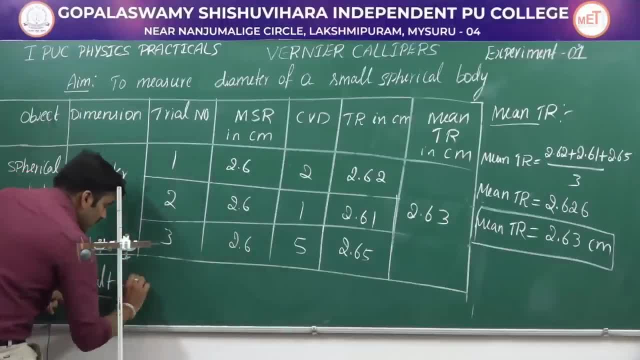 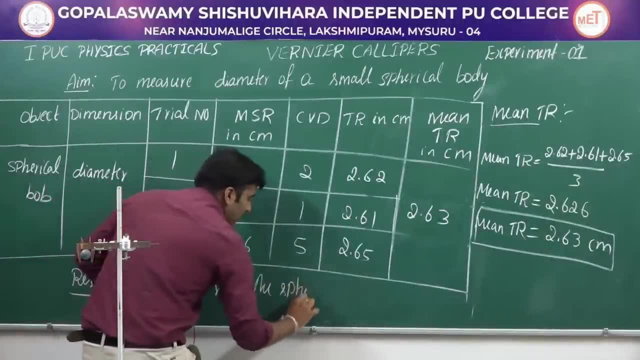 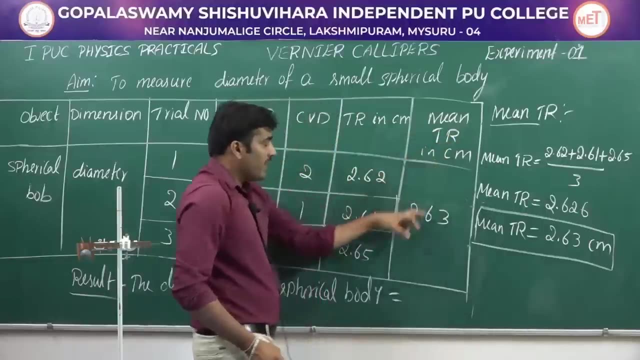 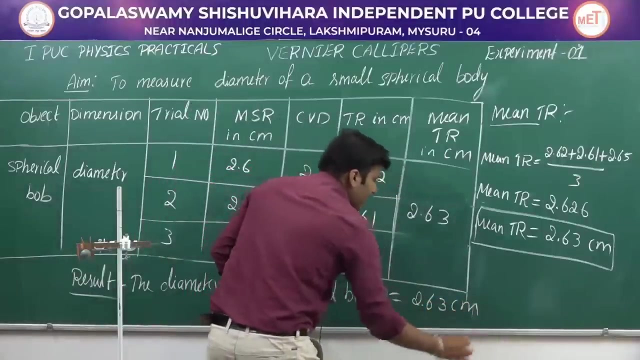 okay, The conclusion of the experiment. The result is: the diameter of the spherical body is equal to. So this is mean TR. So we have to write the value of mean TR for the result. So the mean TR is 2.63 centimeter. correct, This is 2.63 centimeter, But we should keep. 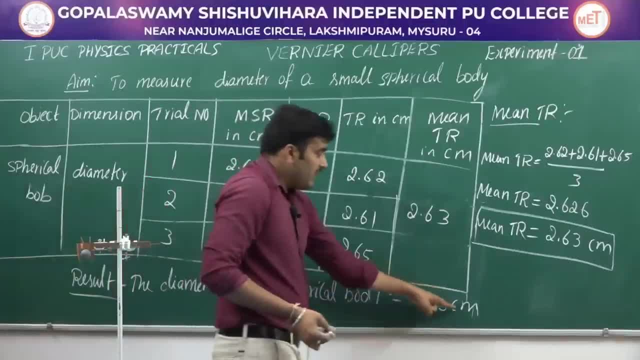 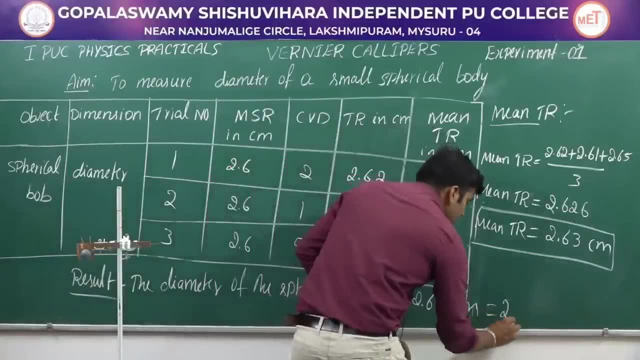 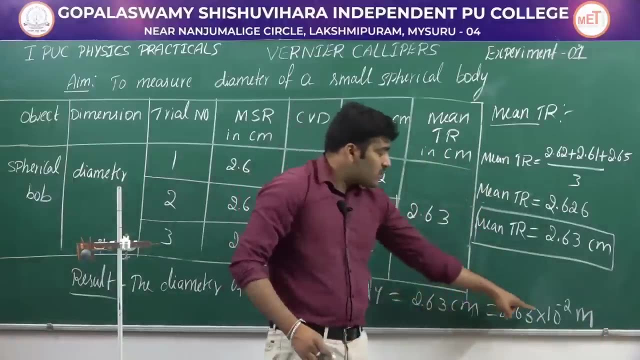 the final result always in a SI unit. So the centimeter is a CGS unit. You need to convert meter into meter. now How do you convert it? This is 2.63 into 10 power minus 2. meter Centi refers to 10 power minus 2.. Therefore, 2.63 centimeter will be equal to 2.63 into.